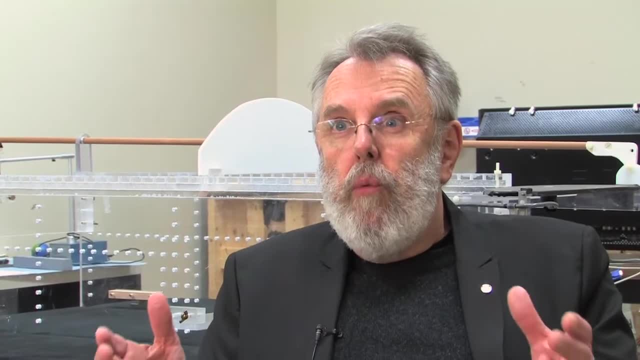 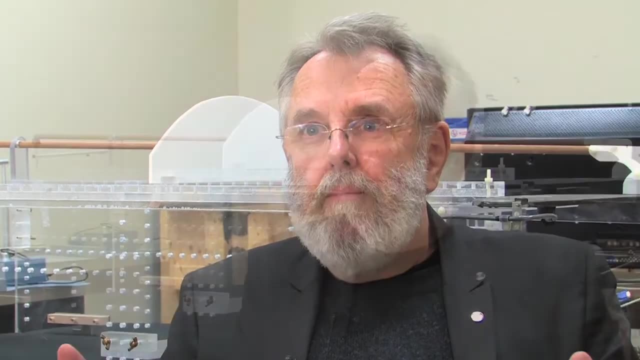 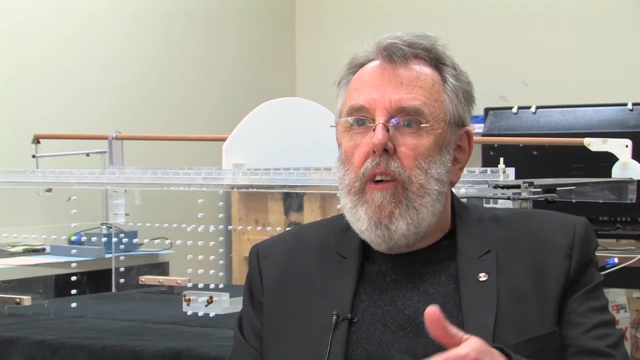 That's called size constancy, and one of the questions we were interested in was: how does the brain enable us to see objects at different distances as being the same size? One of the interesting things that prompted an understanding of size constancy was something called the afterimage. 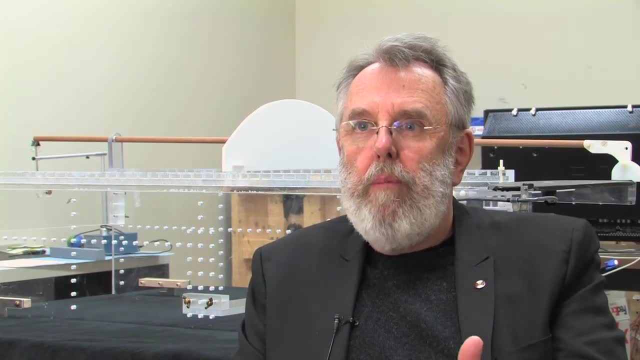 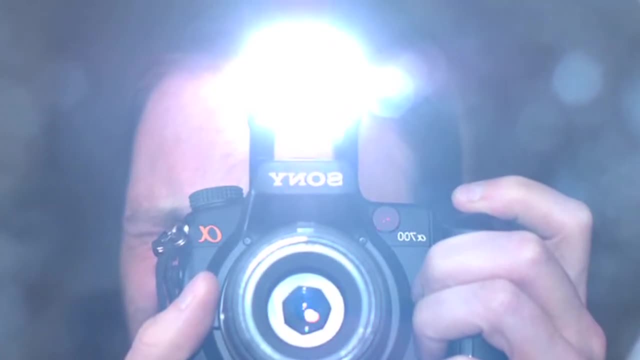 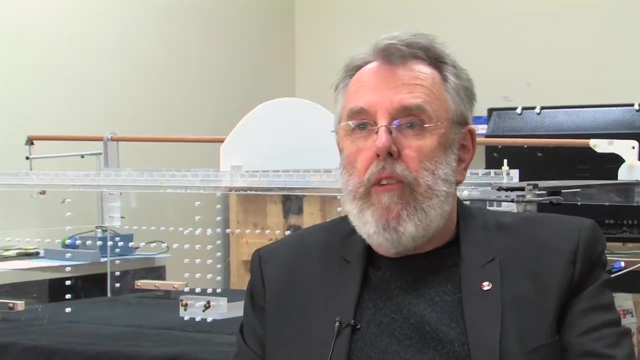 An afterimage is something that we've all experienced. You might be, for example, at a wedding. a flashbulb will go off as someone's taking a picture and that image of the flashbulb will go off. And that image of the flashbulb will stick with you because it excites the back of your eye so thoroughly that when you then look at another surface, like a wall, for example- 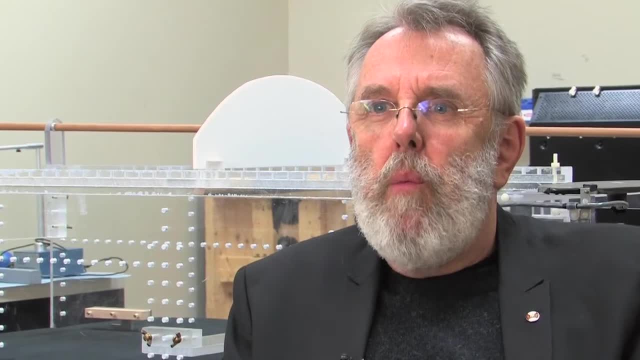 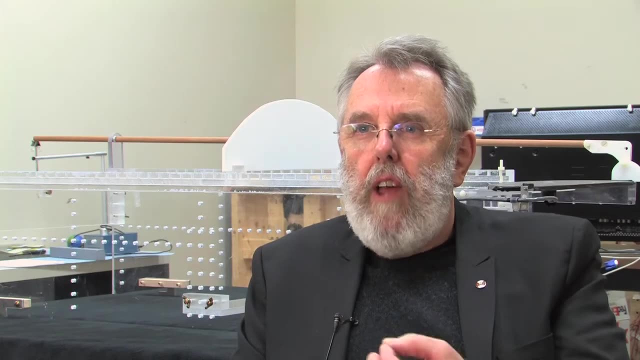 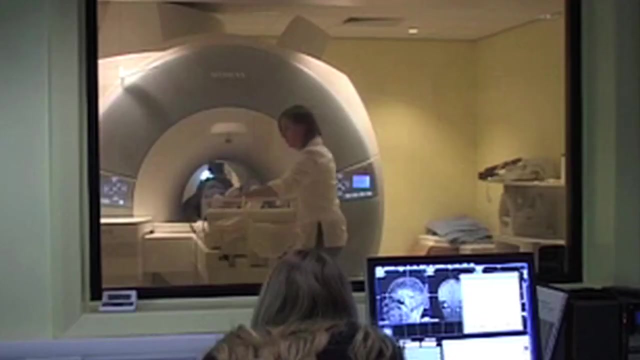 you'll see a rather dark spot where that flashbulb went off. So what the afterimage allows us to do is we can ask people who've got this afterimage set up to look at surfaces at different distances from them while their brains are being scanned. 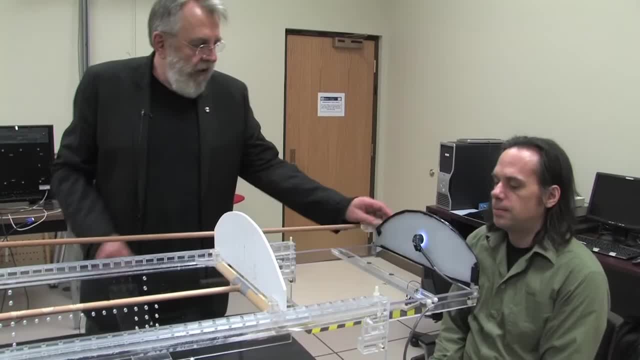 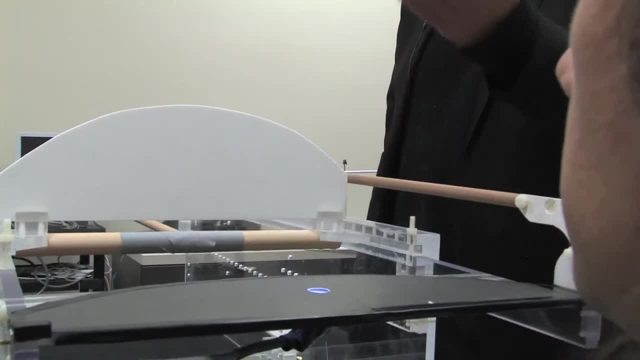 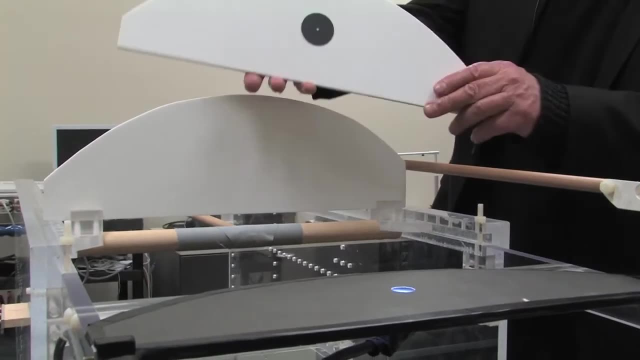 And of course they'll see the object, or the afterimage, rather, that's previously been scanned. is there the same size, And so that allows us to explore the brain and find out how the brain changes as our perception of the size of the afterimage changes. 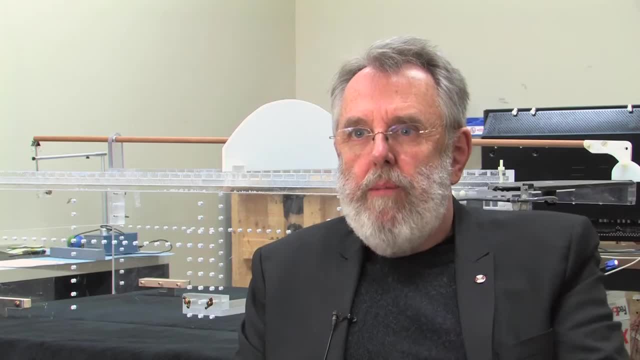 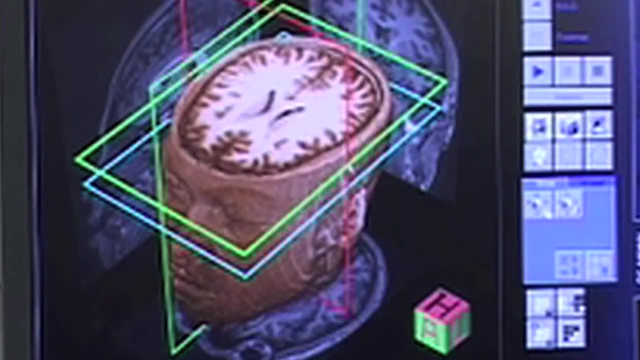 When visual signals from the eye reach the brain, they enter what we call the cerebral cortex. that part of the brain that looks a bit like a walnut And at the back of the head is where the primary visual cortex is, where the visual information first comes in. 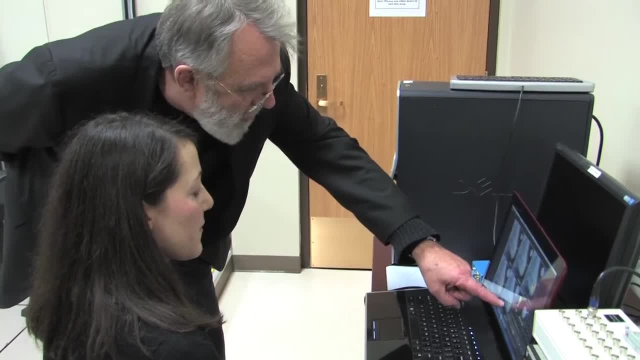 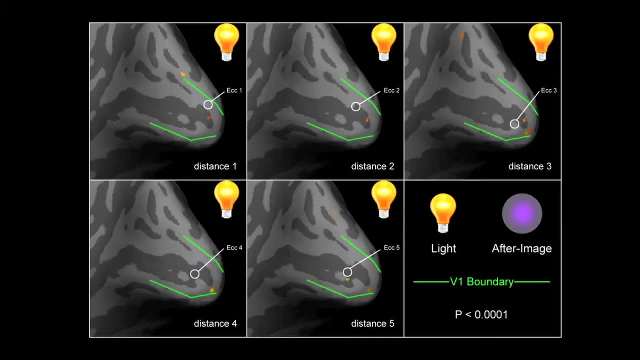 And we know that there's a map of the retina on that visual cortex, a kind of map of the world out there. And so the question that we addressed was: is that map reflecting what's on the back of your eye or is it reflecting what you really see out there in the world?